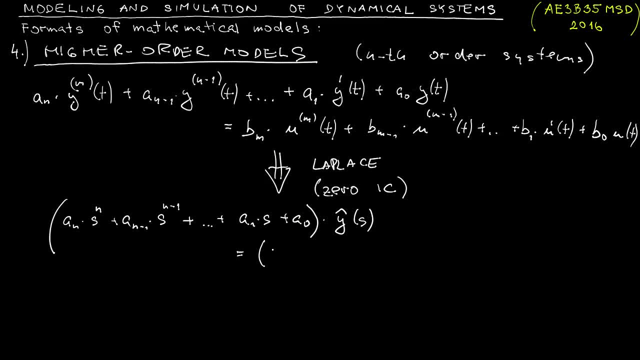 the Laplace transform of the output. On the right-hand side we will have a polynomial again in the S variable, the coefficients b0 through bm multiplying the Laplace transform of the input. Now the culmination of this development is that we can express the Laplace. 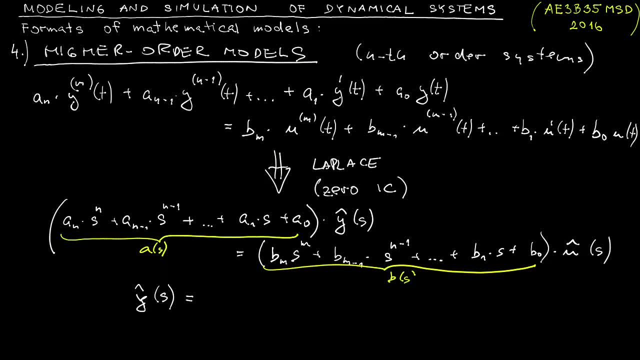 transform of the output as a function of the Laplace transform of the input, using the two polynomials a and b, actually using their fractions. So b over a is the term that relates the input and the output. It's so important that we give it a name. first a symbol. let's label it g and we call it a transfer function. This is a function of the input. 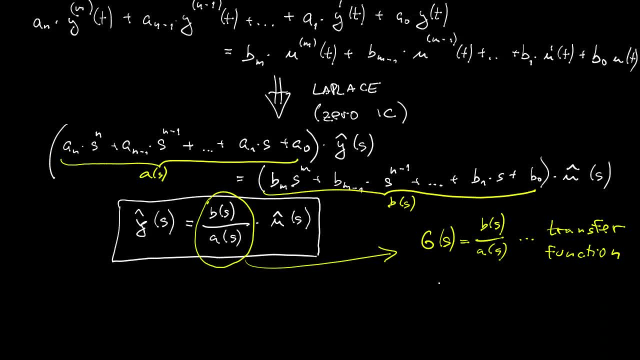 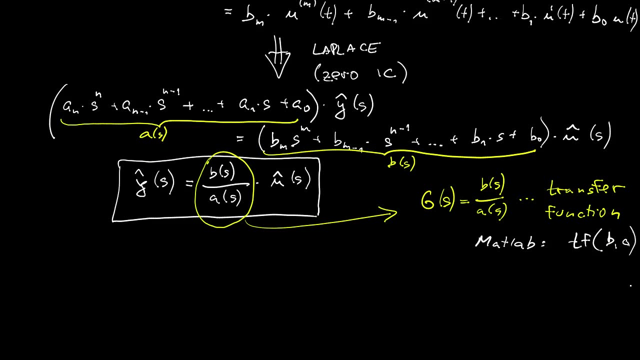 stuff that has been introduced in elementary core or introductory courses on automatic control right now. unless you are familiar with it, you may find it useful to know that there is a function called tf in matlab which you can use to create such model in matlab workspace. now the question is: how does this framework generalize or extends to the situation with? 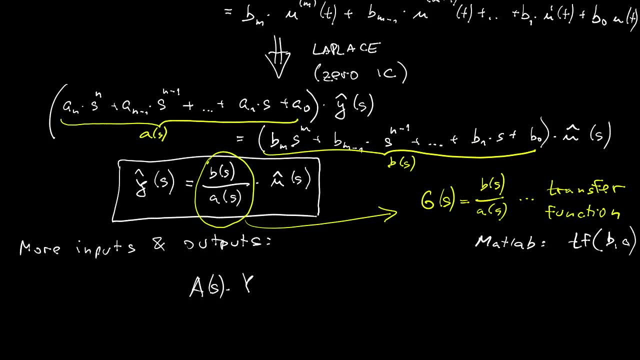 more inputs and more outputs. well, obviously you will have to write a bunch of equations in with time derivatives of several variables. but i will not do it here. it will be quite messy. instead, i will write down immediately the compact version of the of the algebraic equation. so you 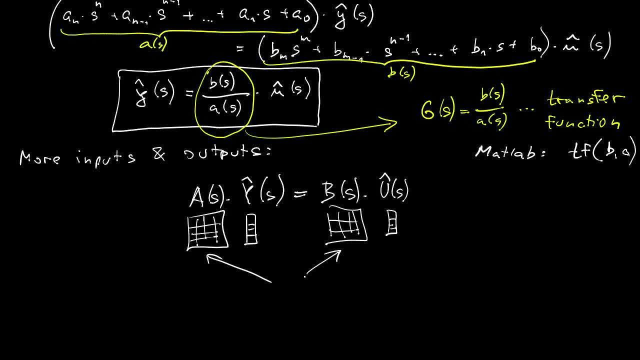 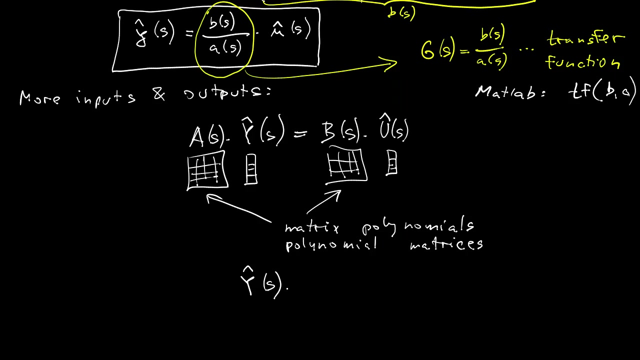 see, on the left and right you have the co, the polynomials, which are actually matrix polynomials. that means their coefficients are matrices. or you can equally well view them as polynomial matrices, that means matrices whose entries are polynomials. now we may be an interesting information for you. well, before first, let's again finish with 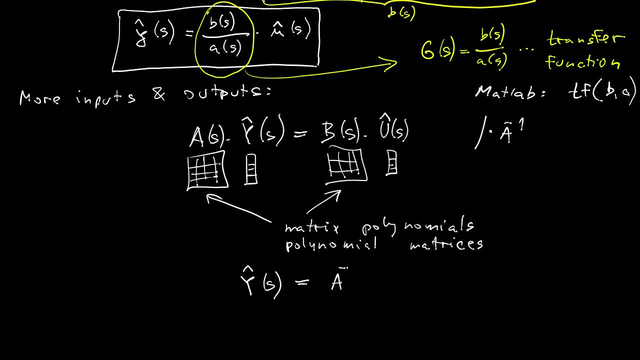 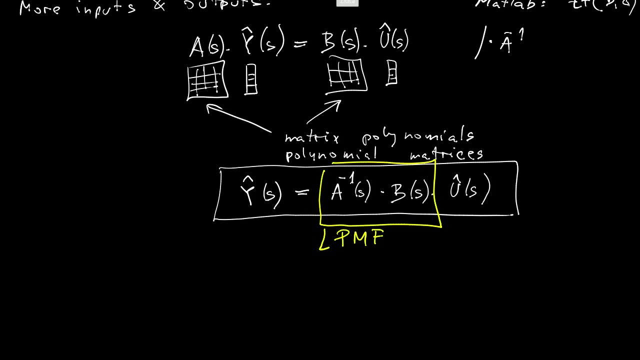 with expressing the output as a function of the input. so we need to multiply both sides by the inverse of a, and what we obtain is again a fraction of polynomials, but this time matrix polynomials, or also called left polynomial matrix fraction. so this is the perfect analog of the.